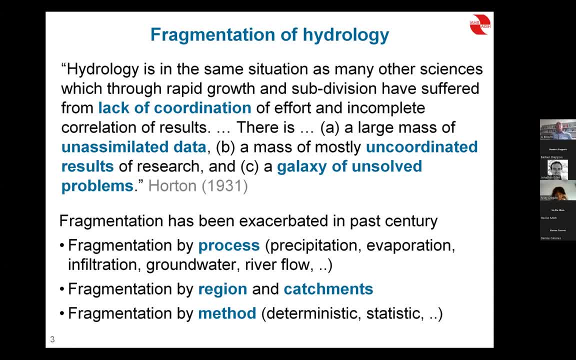 So I was saying there's a certain element of fragmentation, hydrology, and there are not so many studies where all the hydrologists of the world work on one particular scientific problem, but one group calibrates them all in their catchment and another group do their subsurface analysis and erosion etc. with not as much coordination as it is, for example, in the climate science world. 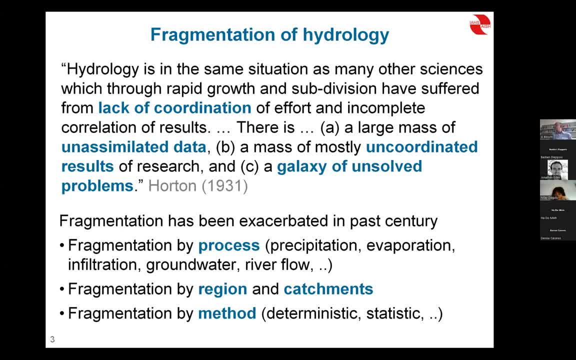 Or in ecology. In ecology, it's very clear: biodiversity is a good thing, so we need to all contribute to more biodiversity. And in climate science also, there's a very clear mission and our mission is more fragmented, which has to do with a number of reasons. One of the reasons is certainly the education We have: hydrology education, geography, engineering, geology, etc. 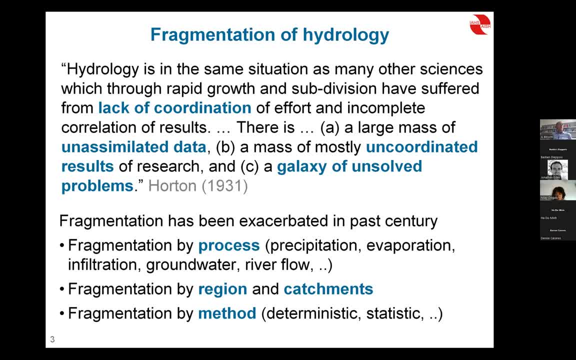 One of the reasons is the education of the people. One of the reasons is certainly the education of the people. One of the reasons is that the hydrologic processes that are interesting for practical reasons are often spatially limited, so it don't span the entire globe. 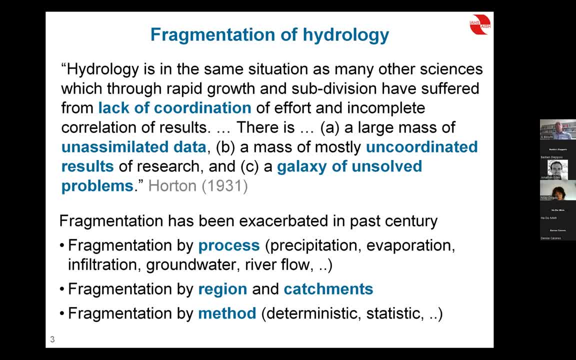 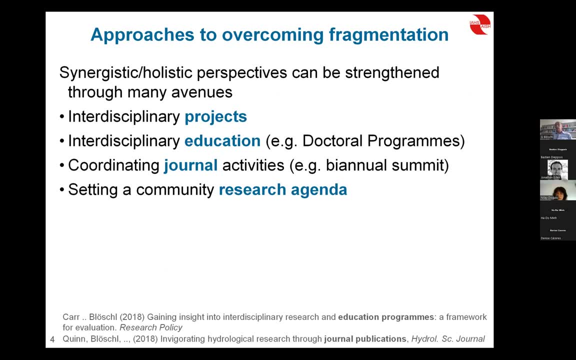 And there may be other reasons that are more cultural within the community of hydrology. So there's fragmentation, as I'm showing here, in terms of processes, spatially, and also in terms of the methods, And I think it would be a good thing to overcome that fragmentation more. 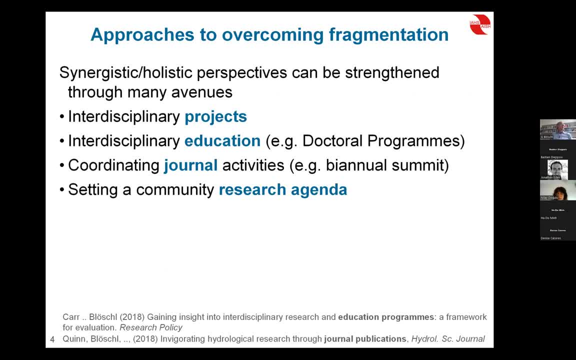 So there's fragmentation, as I'm showing here, in terms of the methods. So there's fragmentation, as I'm showing here, in terms of the methods. There are more synergies, more syntheses within hydrology, And there are a number of ways of doing that: through project, collaborative projects, through education. 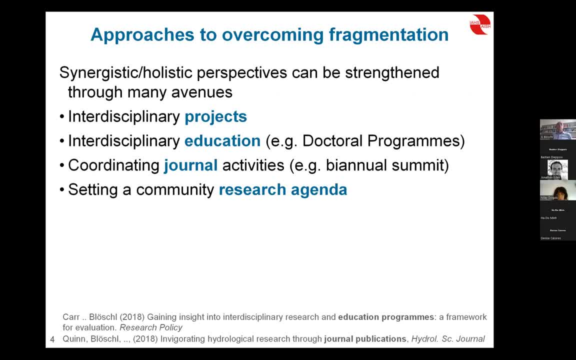 Also coordination of the journals And also setting a community research agenda, And the community research agenda is what I'm talking about today. And the community research agenda is what I'm talking about today: setting a community research agenda. Previous efforts of agenda setting have been more limited. 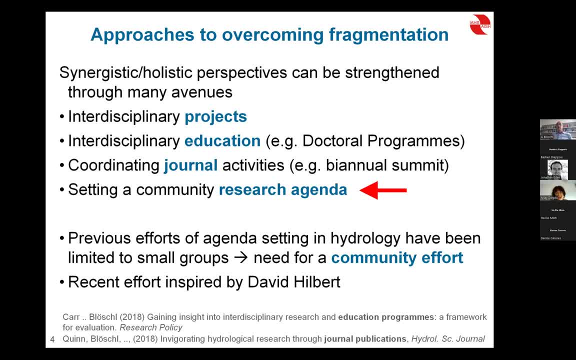 just involving small groups. There have been a number of attempts of doing that, mainly national, not so many international ones- And this particular initiative, UPH- Unsolved Problems in Hydrology- has been inspired by David Hilbert. He was a German mathematician. 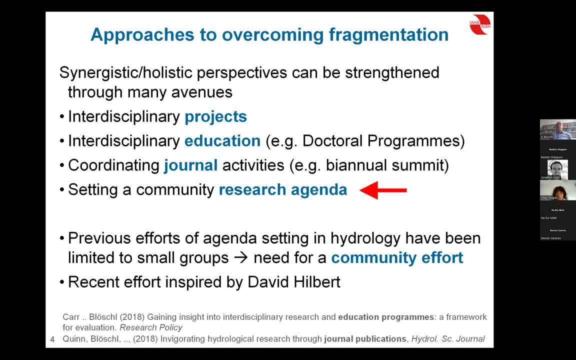 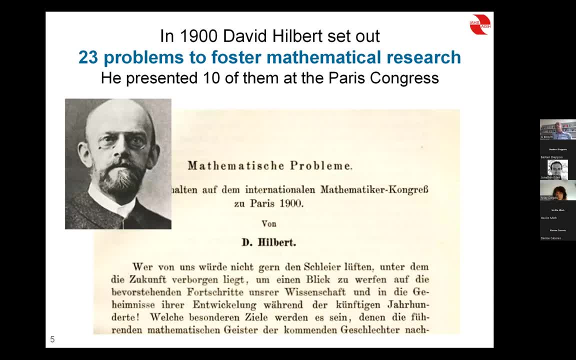 about 100 years ago, He was a genius, And this is this gentleman. And in the year 1900, at the turn of the century, between the 19th and 20th century- he published a paper and presented it at the Congress of Mathematicians in Paris, about 23 unsolved problems in mathematics. 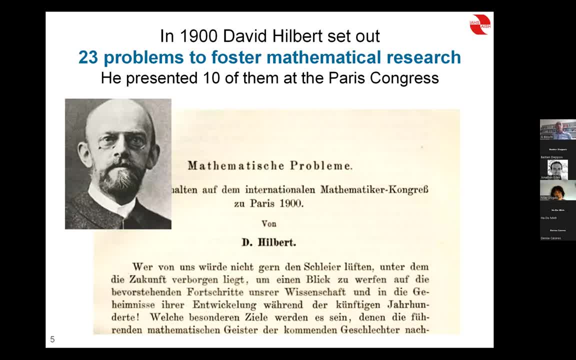 And problems not in the sense is how can we supply water to the city of Paris, But mathematical problems, research problems, proper research problems. And he encouraged the community to work on these 23 problems And this is the reason also why we selected. 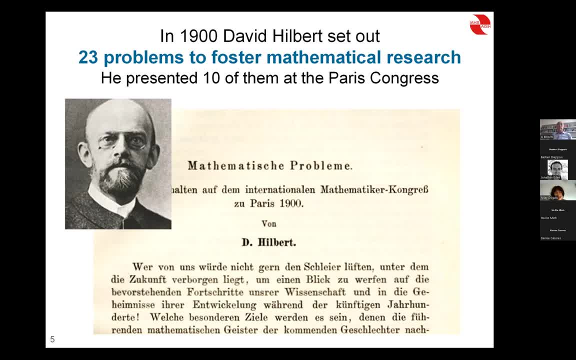 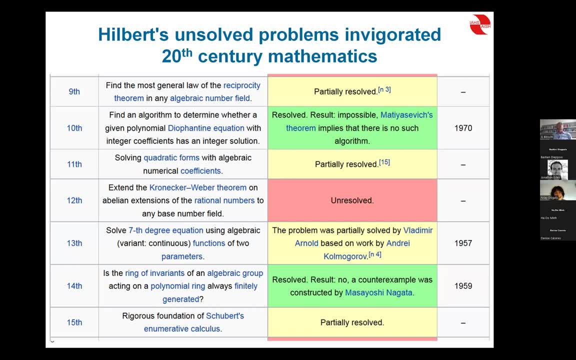 23 for the case of hydrology, But Hilbert had 23 problems. It happened to be 23 problems. Okay, and here is just a copy, screenshot from Wikipedia, of some of the problems that we've been working on, Hilbert's Unsolved Problems, For example, the ninth problem: find the most general law. 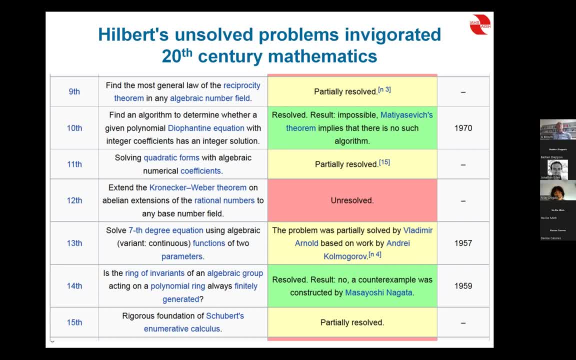 of the reciprocity theorem in any algebraic number field. I don't know what it means, but mathematicians I'm sure will understand that. But the important thing here is the color code on the right hand side. Green means resolved Number 10,, for example, has been 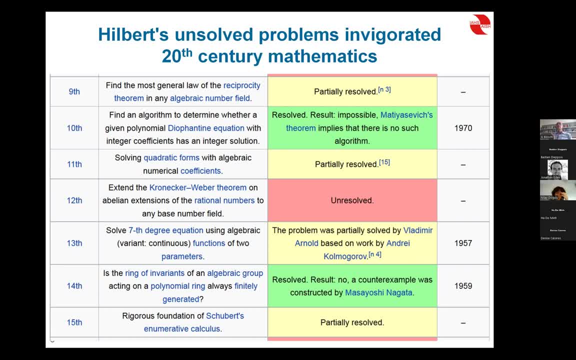 resolved in 1970.. This is 70 years after he had proposed this problem And this problem, this problem And the 12th one is still unresolved. There's still more food for thought for mathematicians, But this is the context, that what has inspired us to do something similar in the discipline. 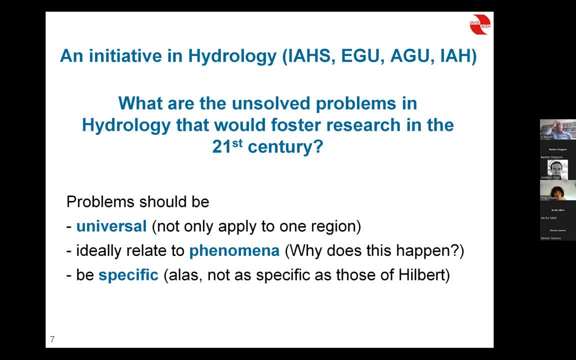 of hydrology. Okay so an initiative in hydrology. What would be unsolved problems in hydrology that would foster the research in the next century? This problem should be universal, So not. what is the runoff coefficient in my favorite catchment? That's not the universal. 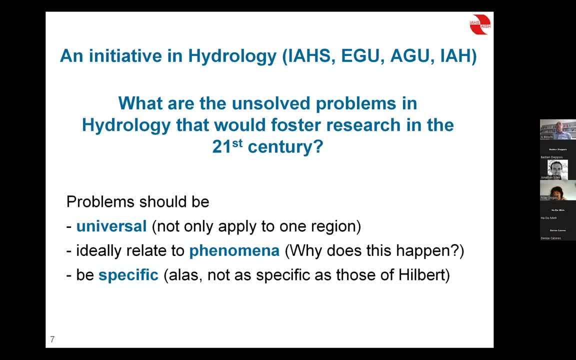 problem, So it should be related to phenomena. Why does something happen Which would be like the equivalent to mathematical problems, And they should be specific, And unfortunately our problems are not as well defined as they are in mathematics, So we usually cannot even 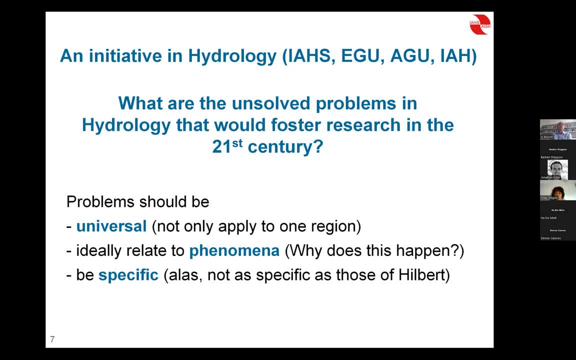 talk about solving a problem- Hydrology- but we usually we address a problem Because boundary conditions are not well defined and catchments are not as comparable as we would like them to be. But still I thought it would be worth an attempt. So, increase the coherence of the community, energize the 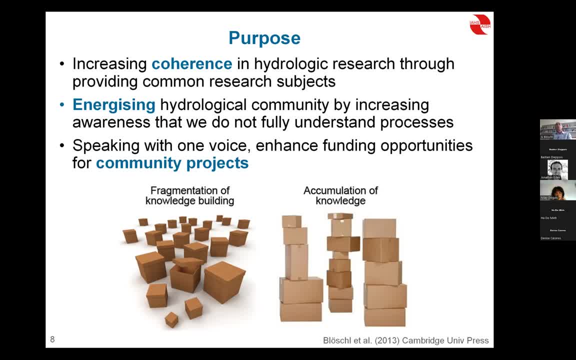 community And speaking with one voice of the three main purposes to go from the fragmentation to the accumulation of knowledge. This is a picture taken from the predictions in ungauged space book published by Cambridge University Press 10 years ago. If you're interested in. 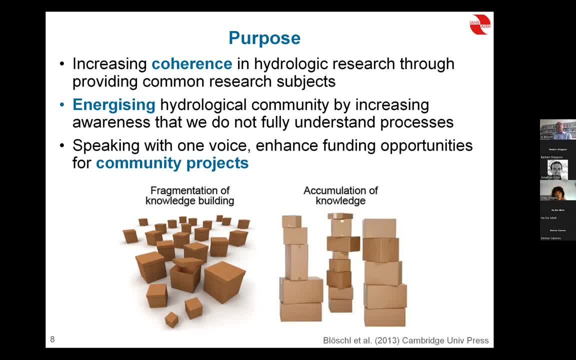 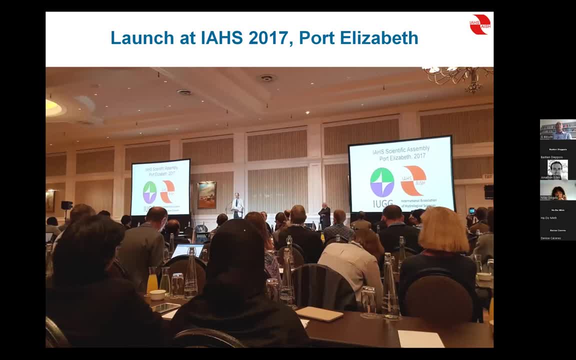 predictions in ungauged basins. this is a recommended reading. I would say Okay. the UPH unsolved problems in hydrology initiative was launched in 2017.. 17 in Port Elizabeth, South Africa, and you can see Hubert Samoneri on the stage and where we started. 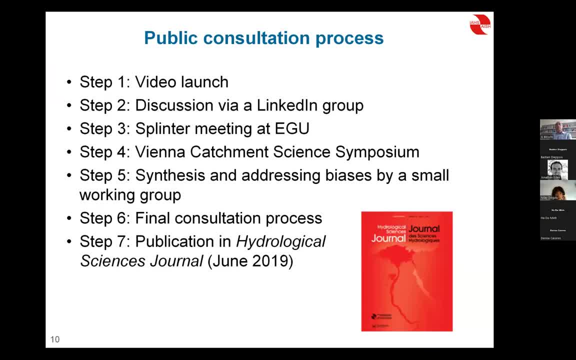 the initiative And we envisaged a a like a workflow of the initiative and seven steps, starting with a video launch that was published on the internet. Then we had online discussions in a LinkedIn group, Then we had number of personal meetings. This was pre-COVID, of course. Then we had a symposium in Vienna. 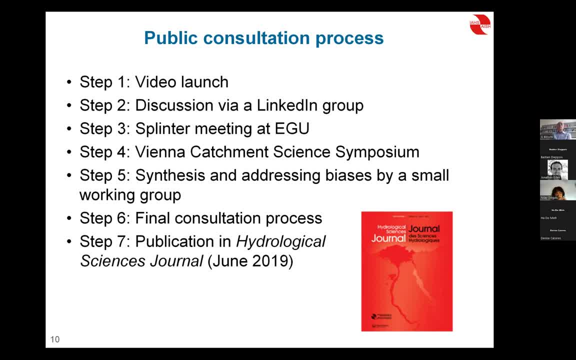 one of the Vienna Catchment Science Symposiums. We have a tradition of running them after each view in Vienna at my university. This year we don't have a Catchment Science Symposium. This year we are running a symposium on the next decade of IAHS, which will be helping 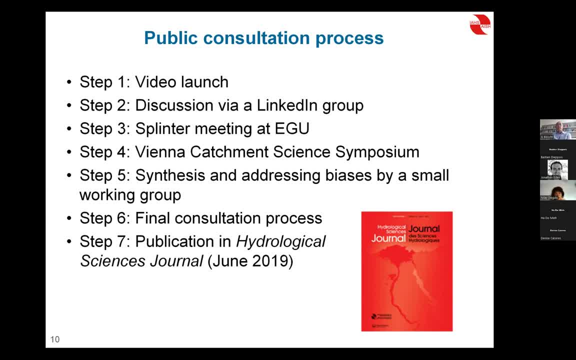 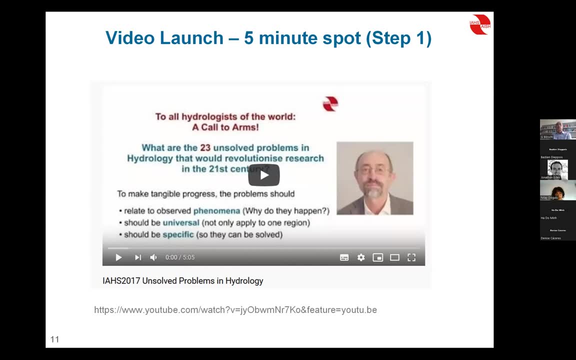 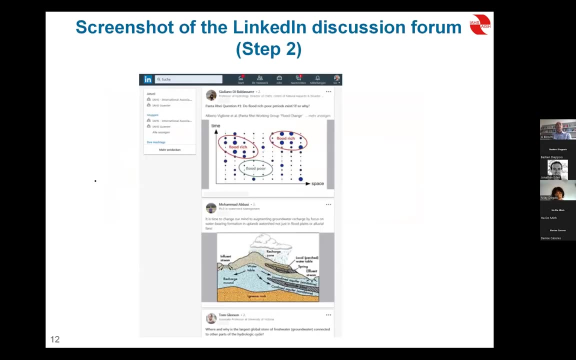 Step five, a synthesis and addressing biases of this discussion process. final consultation and publication as a paper. So these were the seven steps And here's a screenshot of the video launch, just explaining essentially what I'm saying now as a video message, And step two, a screenshot of this. 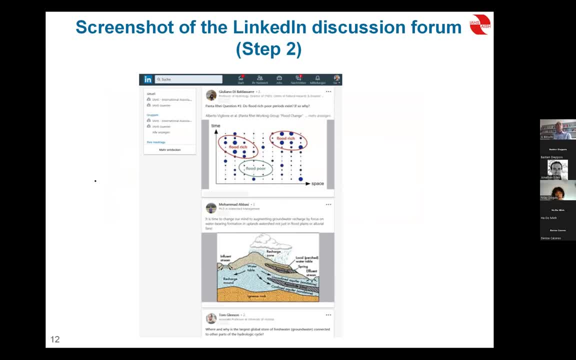 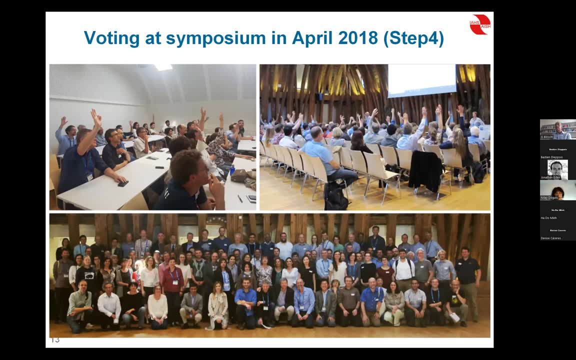 consultation, this discussion process in LinkedIn, And then the physical meetings: two splinter meetings at EGU And this is the Catchment Science Symposium at my university. We had a very good participation, as you can see, And the nice thing- I think that the thing that most participants appreciated very much- is that. 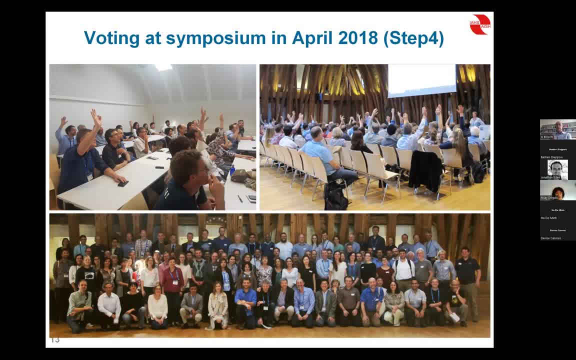 we gave them all the right information and then we voted on the questions. So we had the procedure of classifying the proposed unsolved problems into gold, silver and bronze And then we voted the priority of the questions: whether there should be a gold question, silver question. 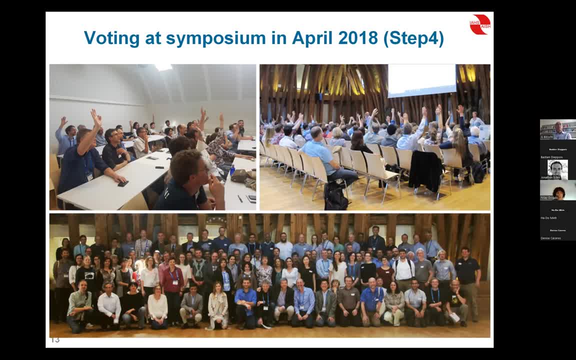 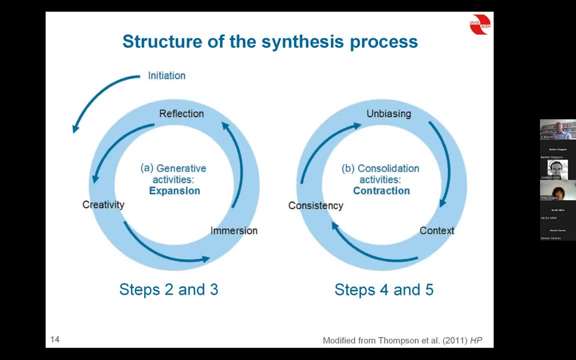 bronze question And we merged some of the questions. we split some of the questions, So this is the voting process Because it's a community initiative. Part of the steps we had generative activities. Generative means creating ideas, brainstorming. 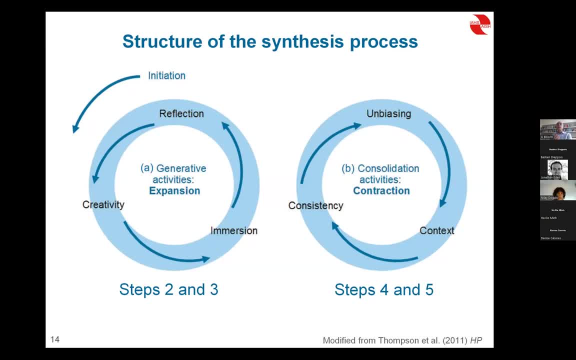 steps two and three, And then we had consolidation activities. contraction, which means brainstorming, is not enough. You want to organize your thoughts, otherwise you are left with a chaos. Both is needed: Creative in creating knowledge, information, ideas. 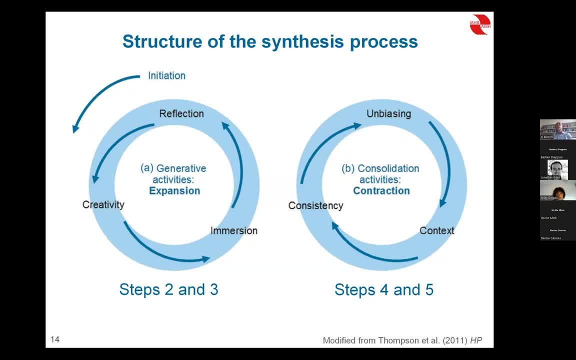 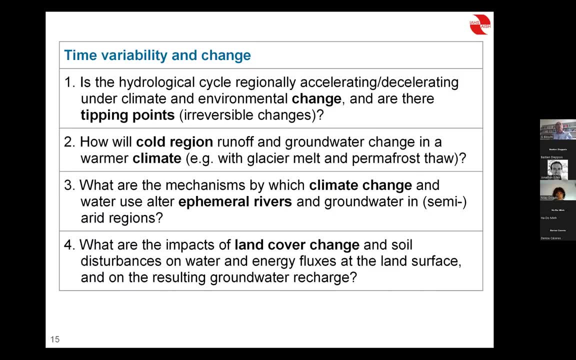 by community, but then you also need to organize them and consolidate them. So we had these two elements in the process And here comes the list of the 23 unsolved problems. We organized them into a couple of groups- 23 into seven groups, seven or eight groups. 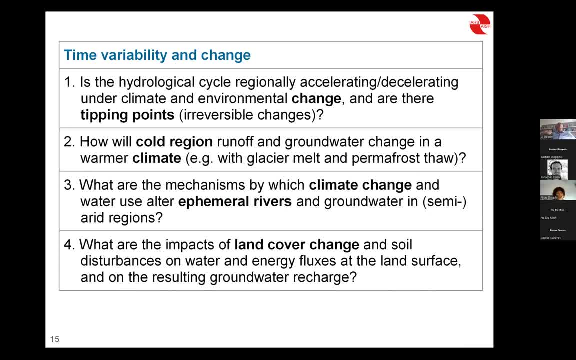 The first one is time, variability and change, And the first question reads: is the hydrological cycle regionally accelerating or decelerating under climate and environmental change, And are there tipping points, irreversible changes? Then how will cold region run off and ground toward? 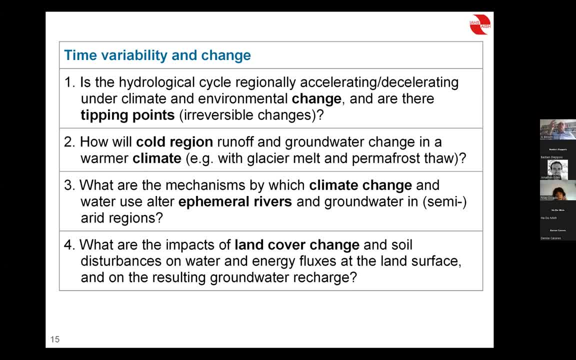 the change in the warmer climate and so forth. So these four questions belong to the group of time variability, And then the idea would be to address more than one group around the world The same question And mentioned even in the journals. this paper addresses science, question number one. 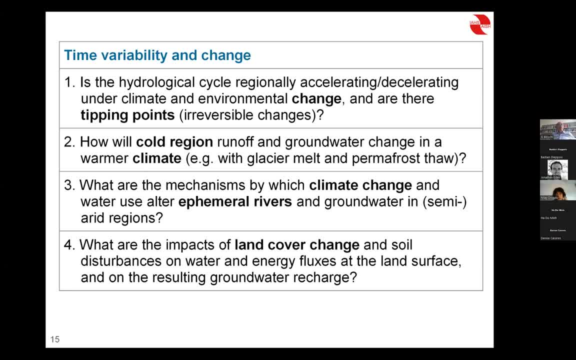 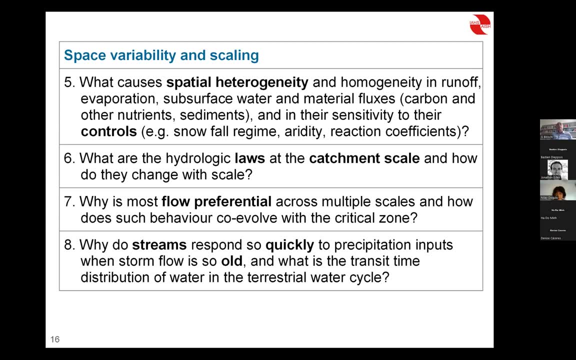 of the unsolved problems in hydrology And then if others read this paper, they can more easily link to the particular findings of that paper. First group: time variability and change. Second group is space variability and scaling. What causes spatial heterogeneity? 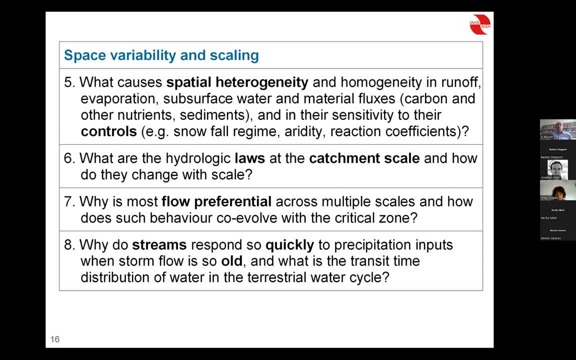 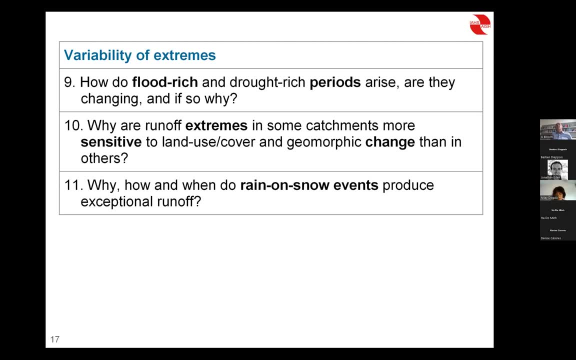 How do we know Catchment scales, law, preferential flow, the residence time of streams? Then we have variability of extremes. Do flood-rich and drought-rich periods exist, and why, Then, sensitivity of hydrologic extremes? And one more specific question: rain on snow events? 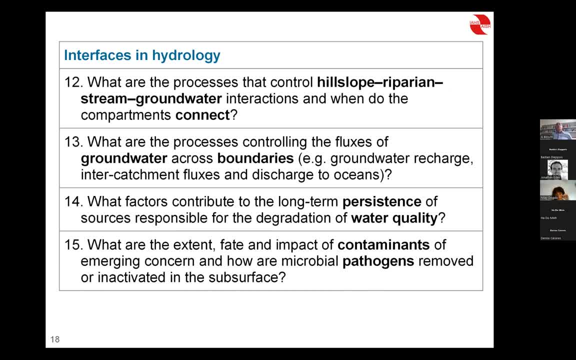 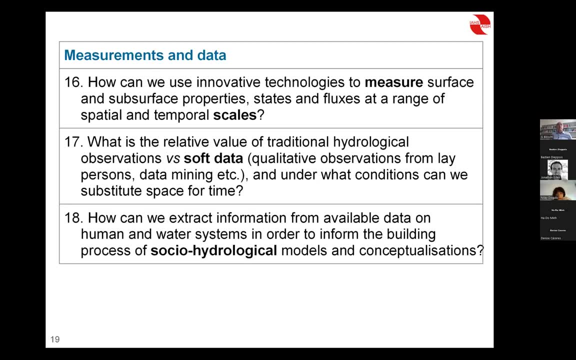 Interfaces in hydrology. What are the processes that control hill slope, riparian stream, groundwater interactions, flows across boundaries, persistence of water quality and the relationship with health? Measurement of data, measurement and data. How can innovative technologies of measurements 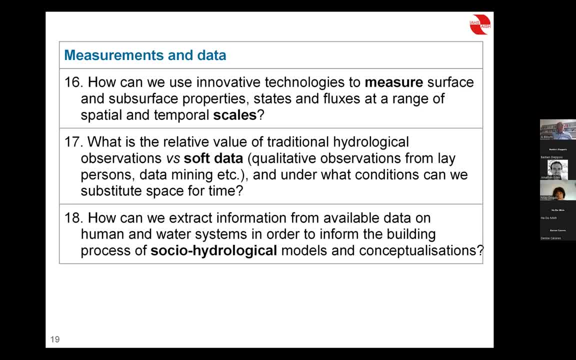 And question 16 is a nice example actually, where you know the initial proposed candidate question was quite specific. It said: how can we measure subsurface fluxes? That was the question And this is a very clear focus question, difficult to solve. 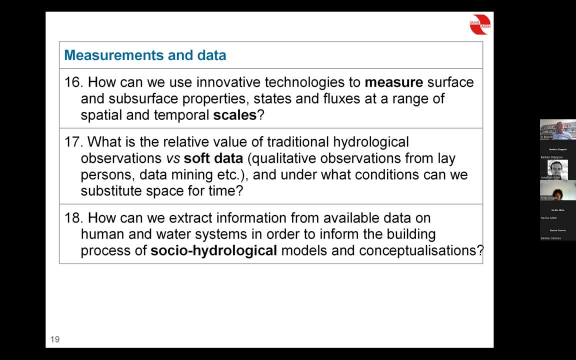 but I think something that would be worth to join forces to further measurement methods of groundwater flux, not just water level flux, not just pressure flux. But then in the discussion process there is a tendency, because of the democratic process, of enlarging the question And so many of the questions turned out to be less specific. 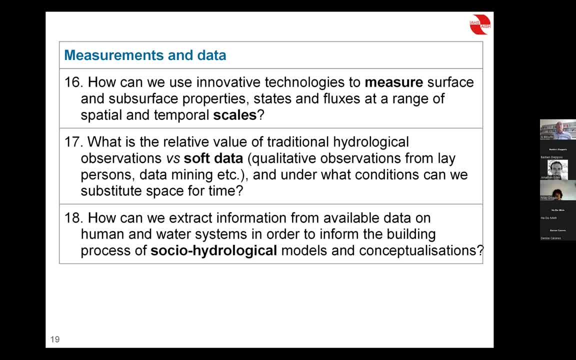 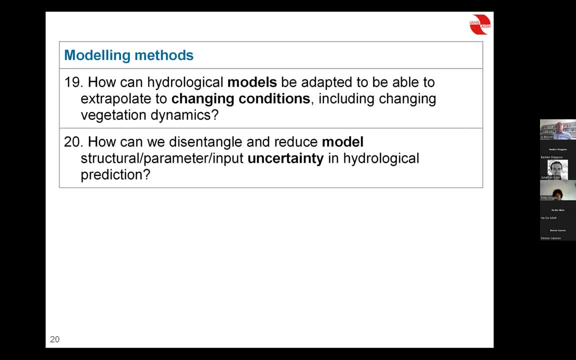 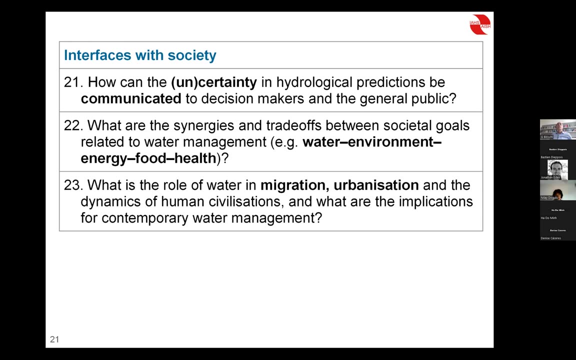 than the candidate questions, And this 16 is an example of that. It's a bit generic: 17, soft data, 18, socio-hydrology. And then we have two questions on modeling for changing conditions and uncertainty. And finally, the final three are about interfaces with society: water-energy-food nexus. 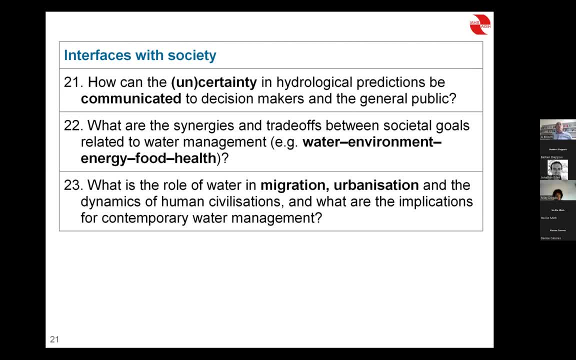 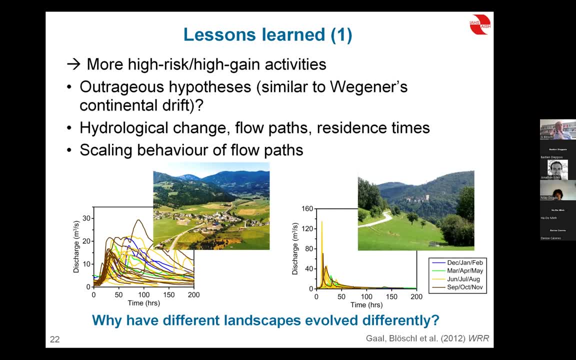 uncertainty in communication, and then something about water and people. Okay, so these are the 23 problems, and I would now like to show you a couple of slides about my personal interpretation of the process and the outcome of the process. These slides are not a direct outcome of this community process, but it's my interpretation. 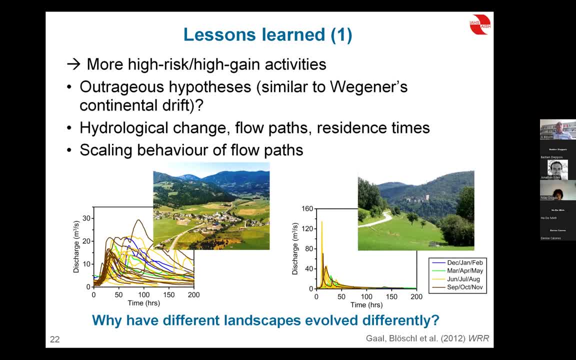 of the thinking that was underway during these processes. So the lessons learned- And one of the lessons learned from my perspective is there is a need for more high-risk, high-gain activities. You may remember, Wegener's theory of continental drift was questioned at the times of Wegener. 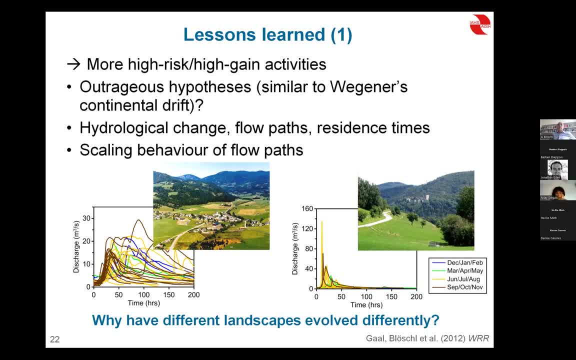 It was not readily accepted. It was initially refuted. It's only after Wegener's death that it was really accepted. Okay, Because it was an outrageous hypothesis. People didn't really believe that the continents would float around on the surface of the globe. 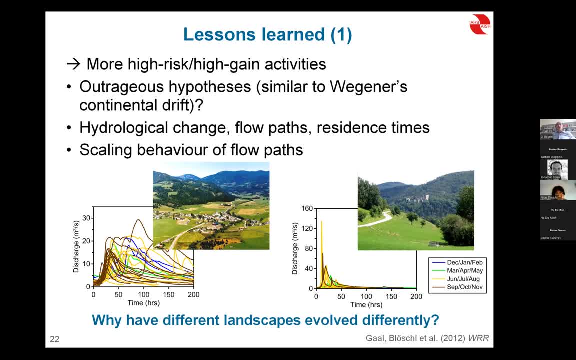 It was unthinkable. So perhaps we need more of these outrageous hypotheses, more high-risk and more high-gain activities. European Research Council is a funding initiative at European scale that actually funds high-risk, high-gain ideas. And the picture shows- And the pictures here are to illustrate- the effect of the co-evolution of the landscape with hydrologic response. 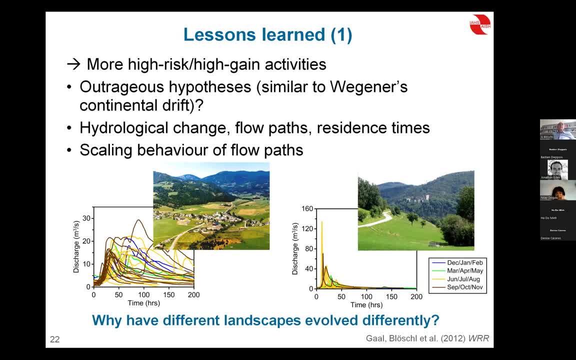 On the left-hand side, a catchment in Austria that has slower response, with little erosion, where the response is dampened and the landscape is flat. On the right-hand side, high erosion, fast response, the co-evolution of hydrology and landscapes. 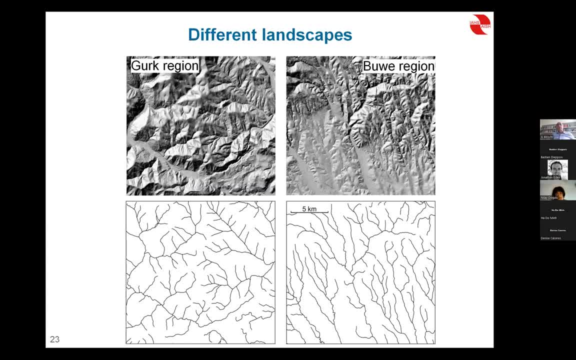 So this is an example, An example of the river network of these two regions. The left one is the Gwerg and the right one is the Buwerk region. Differences in the stream network. difference in the landform has to do with the hydrology. 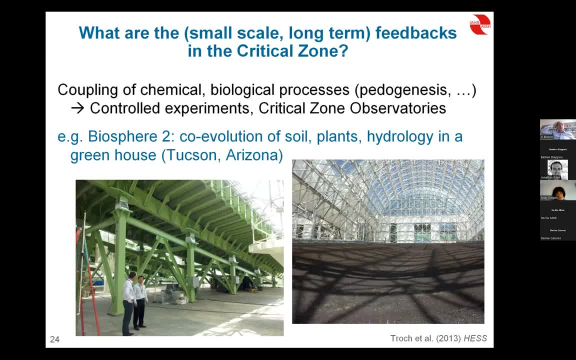 Co-evolution is the topic here. So a question here is: what are the feedbacks in the critical zone? Another of these high-risk questions, And as an example I'm showing here the indoor laboratory of Peter Troch in Tucson, Arizona, where they operated artificial hillslopes undercover in a building and looked at how the soil evolves, with biochemistry and erosion, et cetera. 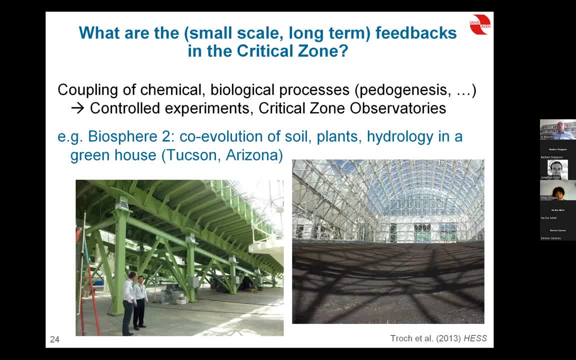 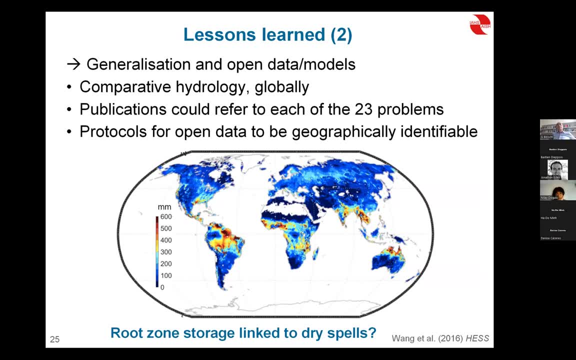 So co-evolution, I think, is an interesting question. Now, another lesson learned is that generalization is important. Open data models is directly related to synthesis, So not everybody should work in their own backyard. We should work better together, including spatially, across different continents, across different catchments. 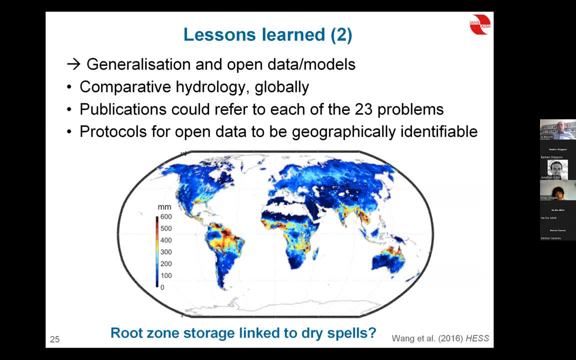 And one way of doing that is comparative hydrology, meaning learning from differences In the hydrology in different places, And publications could refer to one of the 23 provinces, as I mentioned already. and open data, I think, is one of the keys to a successful cooperation, and there are already some initiatives underway for making hydrological data of different countries available globally to all the hydrologists of the world. 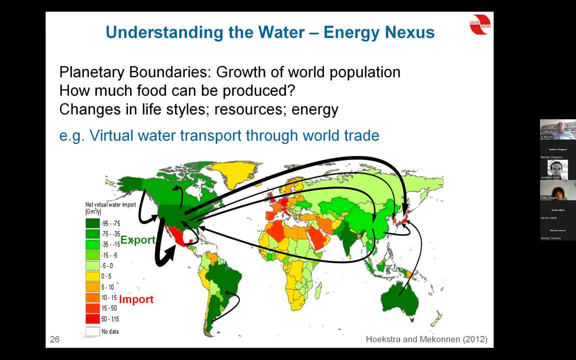 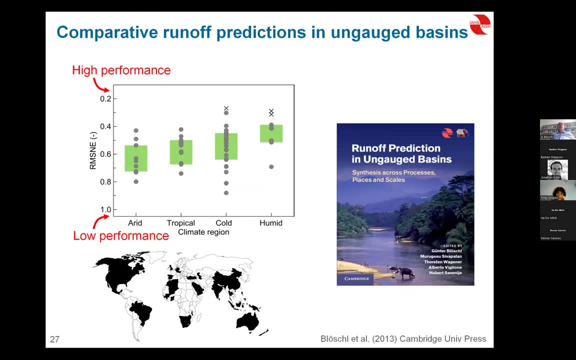 So, to put water-energy nexus, an example again of a global scale analysis, Planetary boundaries, how food, water, energy interact in global scale perspective. And here is an example of comparative hydrology to encourage this synthesis across processes, places and scales: 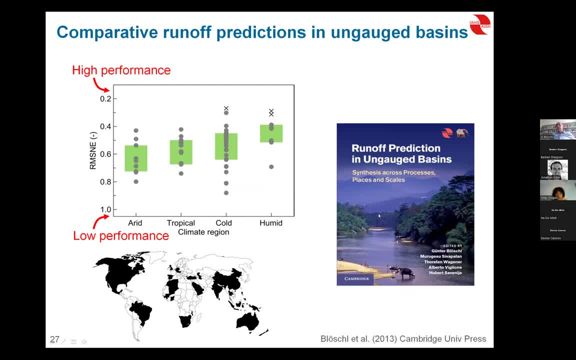 You see here the title page, cover page of the Pap book run of predictions in on gauge basis synthesis across processes, places and scales. an example of this comparative approach of the performance of runoff runoff simulation in different parts of the world. so these black countries are. 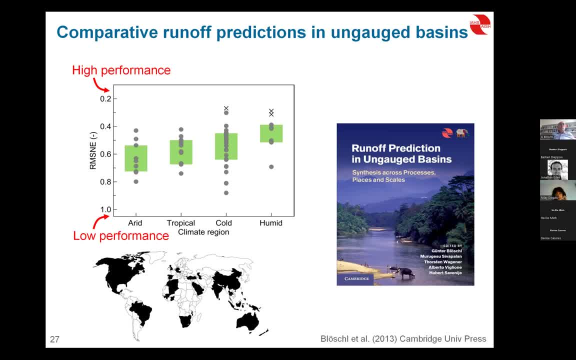 countries from which data has been used to compare different methods of predicting streamflow in catchment, where we have no measurements stratified by the climate- Eric: tropical, cold, human. as you see, as we go from Eric to human climates, The performance of the models increase. this is not the finding that applies to one particular. 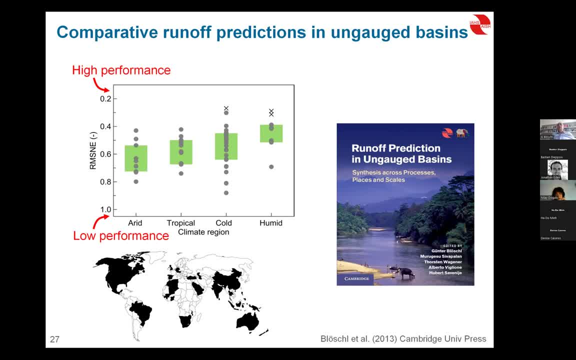 catchment. it's a global finding. this is a kind of funding that unifies the entire Community, at least part of the Community that is interested in this kind of predictions, but globally, not just in one country, and this is the central point here. 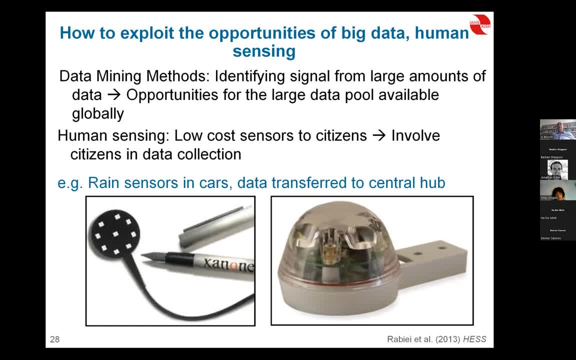 Then slide about new data. big data, human sensing for citizen science is also a very timely topic and that has a lot of potential data mining methods, New technology: this is an example of the rain Center that was developed, I think, in Germany. that is low cost, so it costs a couple of euros and that can be. 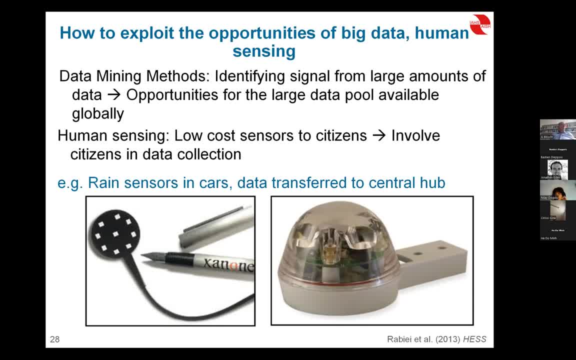 multiplied. so we can, we can use many of these things as thousands, hundreds of thousands, because they are so cheap. one of the many ideas, but therefore many different years, of innovative data and of citizen science that do not necessarily necessarily follow the tradition of hydrologic measurements: few gauges, few instruments, very expensive. 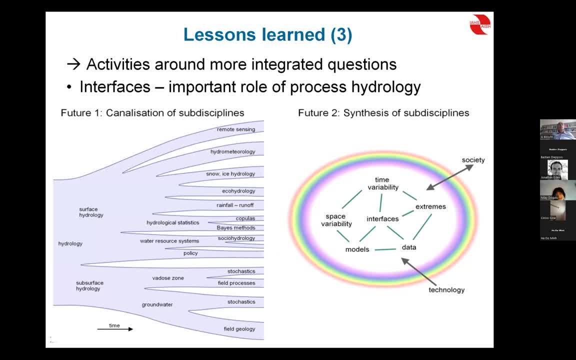 but they also other possibilities. Okay, let's learn three about this, about the synthesis. the figure on the left shows a rendering of the perception of how hydrology has evolved in the 20th century. so at the beginning of the 20th century most hydrologist would say 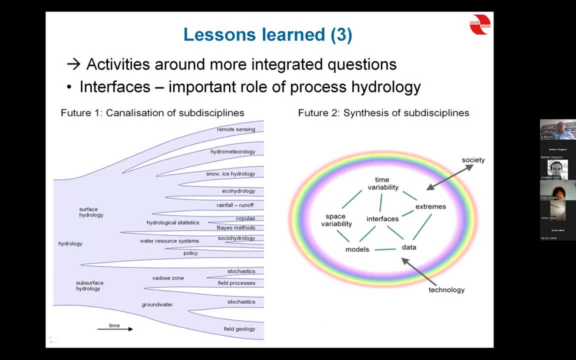 I My feedback of expertise is water, water engineering or science of water, and may even geotechnics, so the most expert at a very broad expertise. and over the course of the 20th century we got more specialized, which is of course very understandable because our knowledge base increased exponentially. so we 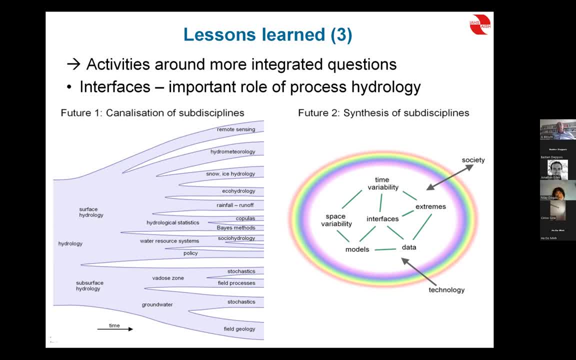 have much more information now than what we had 20 years ago, 100 years ago. but then there is also a risk of a certain fragmentation. some people only working remote sensing, some people on the on the caustic, some people doing just feel people and saying: 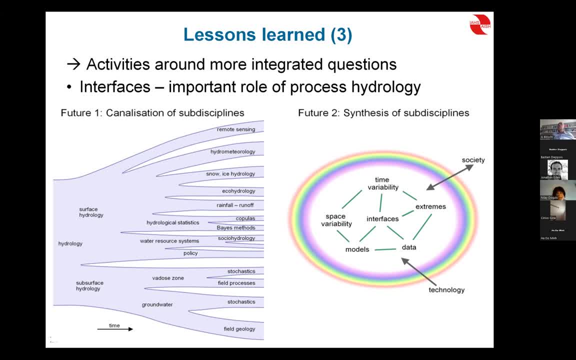 well, we have been people, you are models. we need to collaborate, but to my mind, this is the wrong approach. to my mind, we should. we should all have a broad view. in hydrology, it is we should. Of course, we should be specialist about. 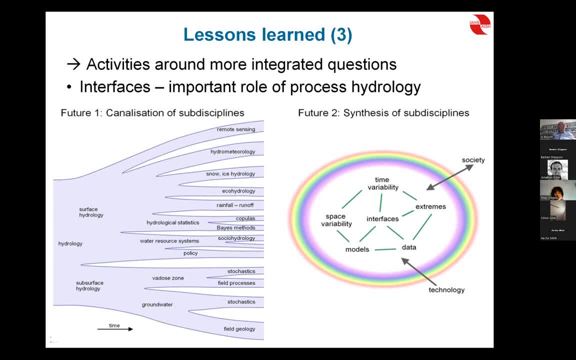 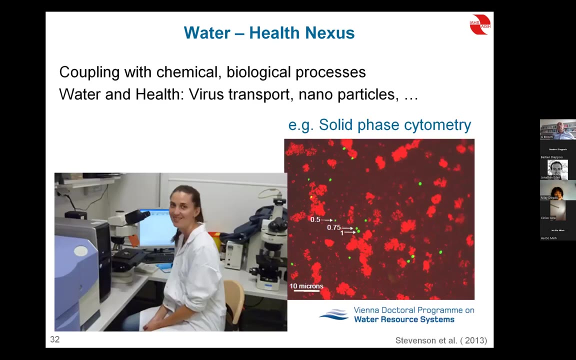 One thing, One particular method. you all have our pet methods, but have enough enough breath to also embrace hydrology as a whole. so this is a vision of hydrology that is more synthetic, not so much split into individual branches. Okay, then I slide about water, health nexus, I think what the health is, a topic that will 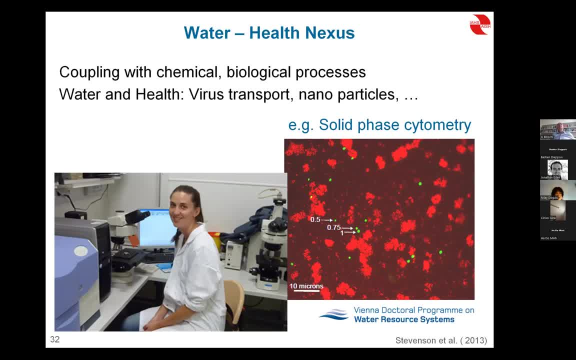 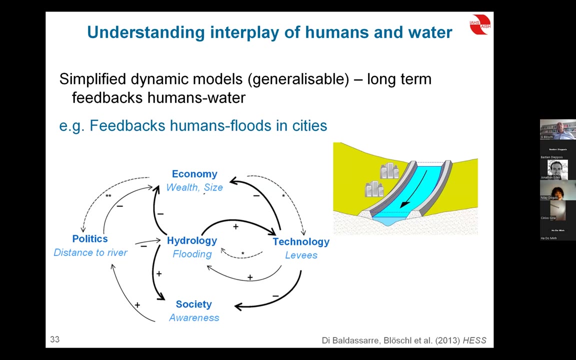 increase continuously in importance as health is becoming more important As humankind is aging. slide from my own doctoral program I'm running in Vienna. there's a group working on water and health- One of the former students here, Margaret- And a slide about social hydrology: interplay of humans and water. 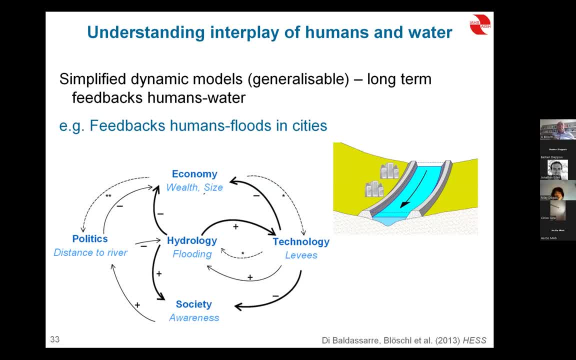 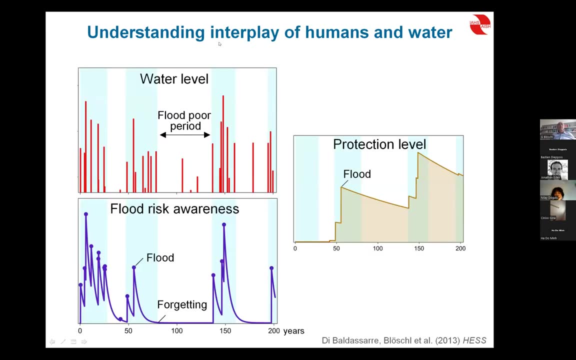 A course, a loop diagram that represents a simplified representation of the feedbacks in the system, in this kind of feedbacks of humans and floods, from a long term perspective. again, a broader view And some examples of that that we not only can simulate water level but we can also. 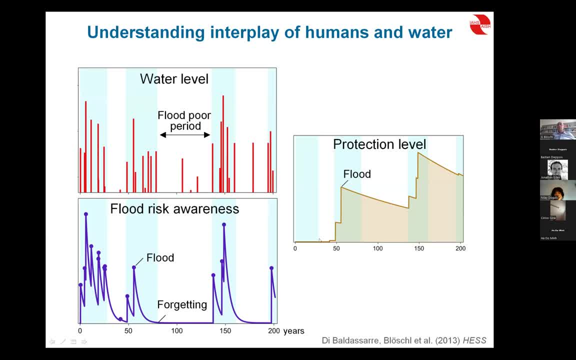 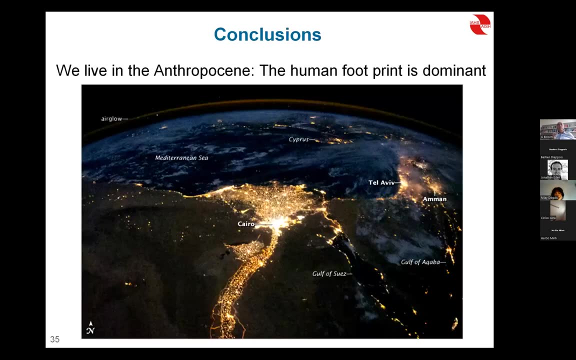 simulate the flood risk awareness of the people and we can simulate to which extent people will some likelihood build dams in the future Or retain water in the landscape. That's a broader view And I think also timely for the 21st century. Okay conclusions: we live in the Anthropocene. 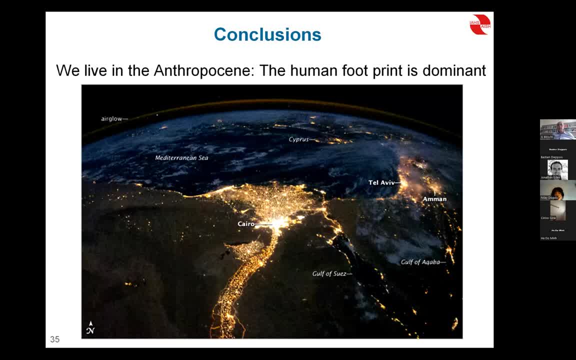 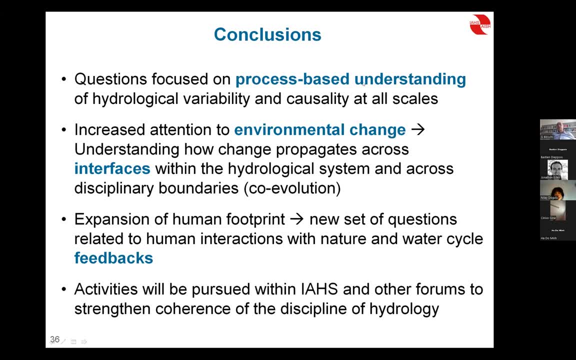 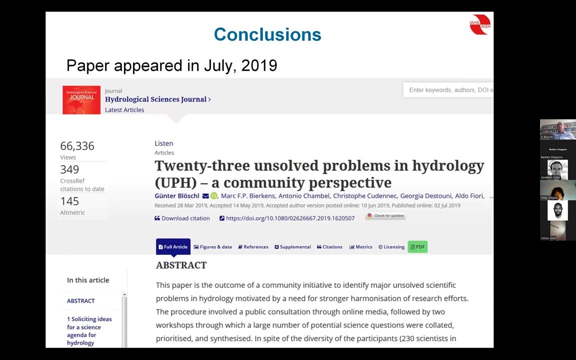 so the topic of change was, of course, paramount in the entire UPH initiative. All the questions focused on the process based understanding of hydrological variability and causality, Increased attention to change and interfaces feedbacks- central to all of that. And okay, and that this is a screenshot of the paper that was published 2019,. 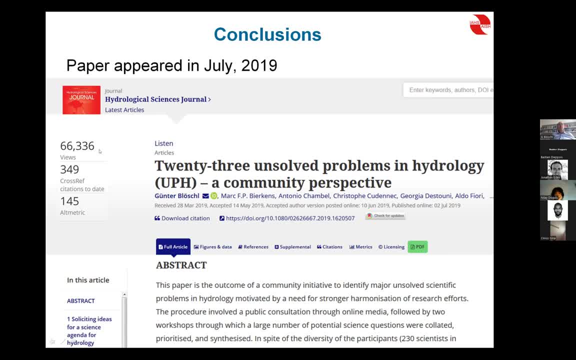 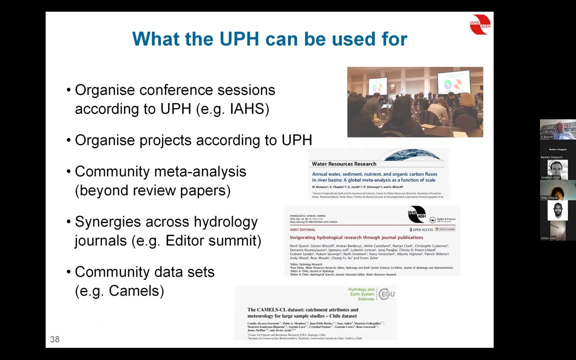 almost four years ago And, as you can see, it has already more than 60,000 views, 350 citations and a long list of authors. So what is it going to be? It's good for now. the question is, of course, that how can it be used? 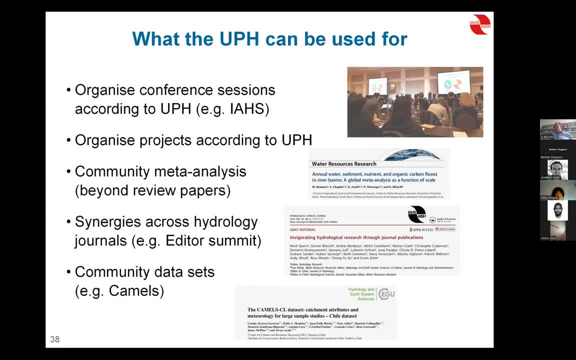 COVID had a bit of an incision on the sharing and the distribution of the results of this initiative because COVID started just at the end when it was published the paper. that interrupted the dynamics of this initiative a bit, but it's now slowly taking pace. 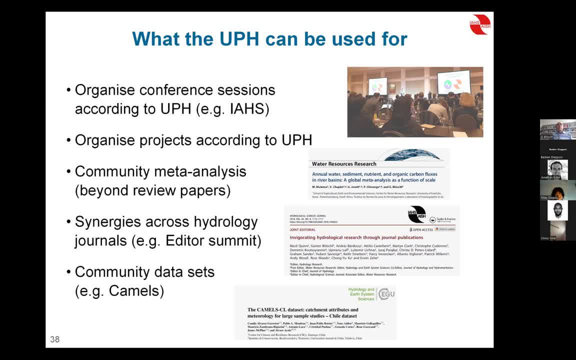 And so it has to be climb up? If so, and what are the alternatives? So I am going to give my observations now. As I say, this is like a prediction. Thanks, Thank you. Read us your thoughts as it is. isn't just the brain, brain. 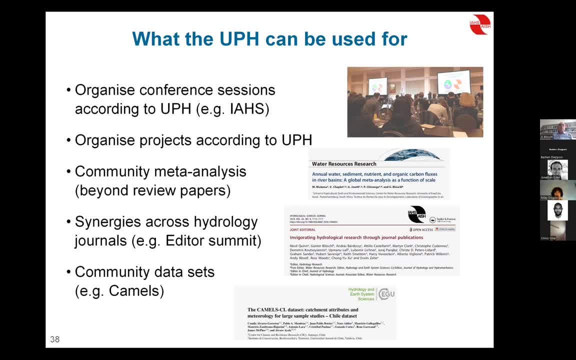 Second, organize projects according to UPH, and some people are already doing that. So saying my project proposal is about one particular science question of UPH. Then the third point here: community meter analysis. So here's one example of my own publication. 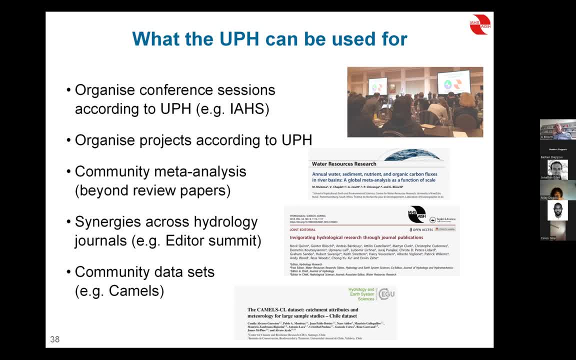 with a group in South Africa. Community meter analysis, I think, is something that is not very hard to do and we do not have a very good tradition in hydrology of doing that. Other disciplines, for example the medicine or ecology- 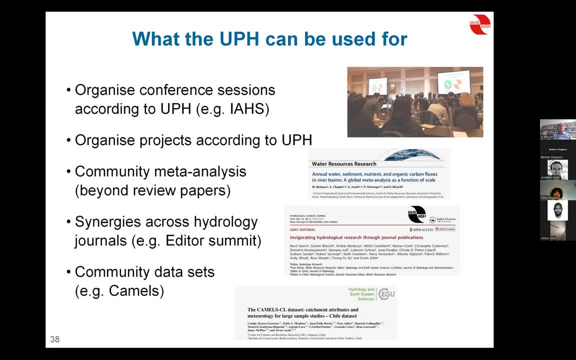 have a much stronger tradition of doing meter analysis, where there is a regular tradition, like every year, every other year on one particular topic, of pulling together all the knowledge that exists on one particular science question, The role of one particular medication, the success of one particular method. 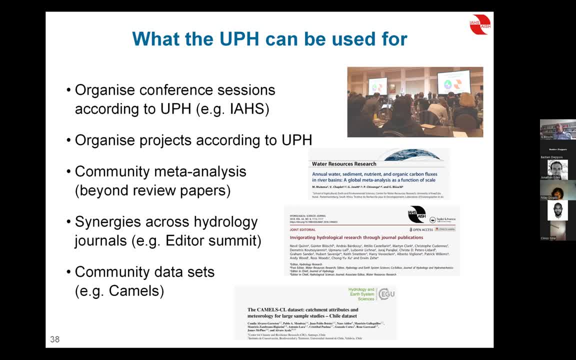 We have a weak tradition of doing that and I think this would not be hard to do. It requires a lot of thinking. It doesn't require so much money. It doesn't require material and funding for fieldwork and data analysis- not so much, but going through the literature. 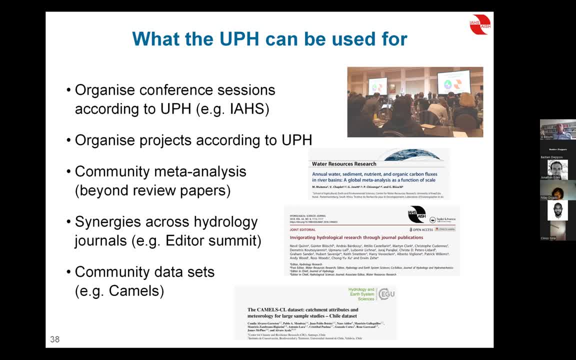 it requires a lot of thinking and talking with each other to find what is the community consensus based on evidence published in the literature on particular questions. So one idea would be: meta-analysis of UPH number one, meta-analysis of UPH number two, etc. This would be an idea. 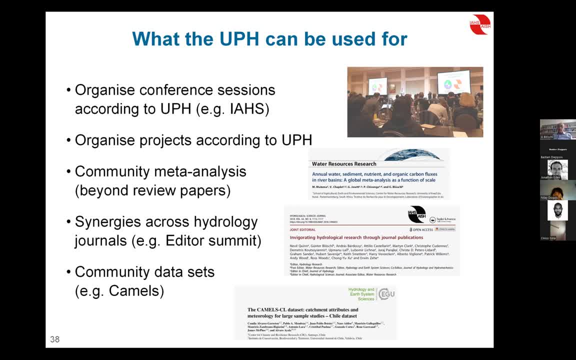 I think it would be worth pursuing and would very much strengthen hydrology. Then, an initiative I have myself been leading over the last 10 years, all contributing to the synergies of hydrology, because UPH is only one of the initiatives I've contributed to enhance the compaction and the cooperation within hydrology. 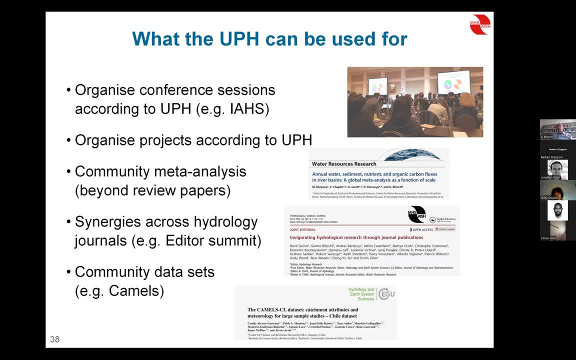 So this particular initiative has to do with our journal publications. I've been organizing meetings on editors of hydrology journals across all the publishing houses. There are a total of 20-25 hydrological journals at the international scale, And so I invited the editor of these 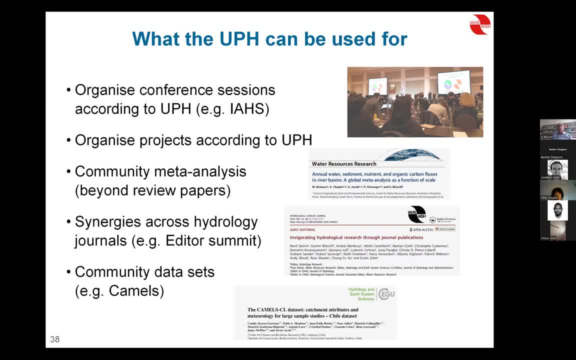 journals and we had meetings every two years And some of the meetings we published a joint editorial as an output of these meetings. This is one of them And that conveys the message of the editors, how the editors feel the potential of the community from an angle of the.